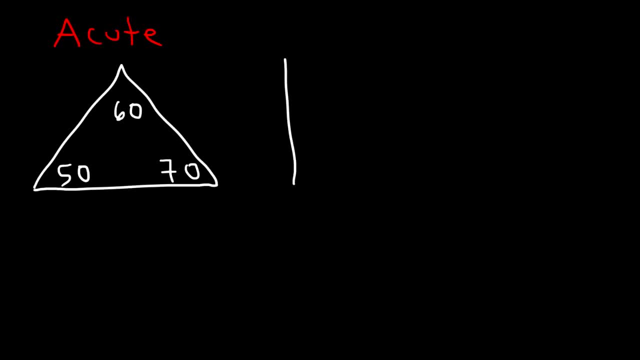 angle that is less than 90.. The next type of triangle that you need to be familiar with is the right triangle. The right triangle contains one angle that is equal to 90 degrees. It's the angle represented by the blue box. Now the 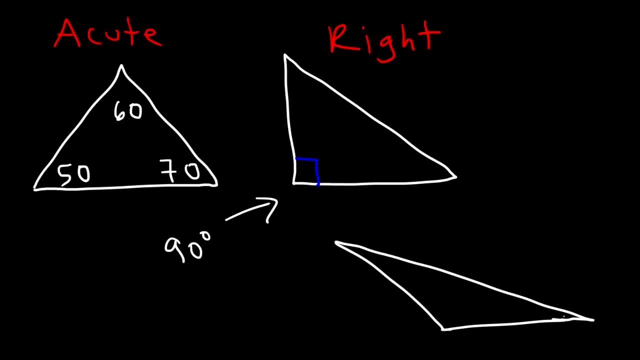 third type of triangle that can be classified by angles is the obtuse triangle. In an obtuse triangle, one is of the angles is greater than 90. so make sure you can classify angles based on- I mean triangles based on the angles. now sometimes you can classify triangles. 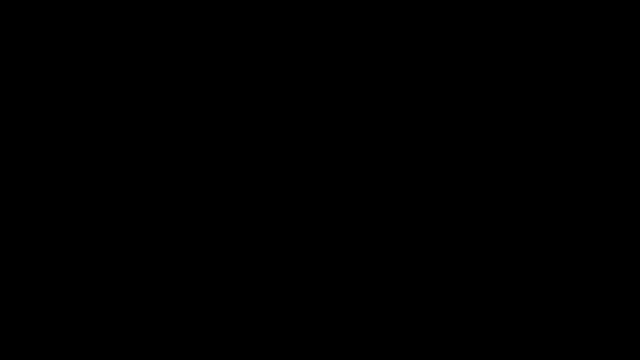 based on your sides. the first triangle we're going to talk about is the scaling triangle. this triangle has no congruent sides. all three sides are just different. the next triangle is the isosceles triangle. in the isosceles triangle, two sides are congruent to each other. the next one I need to be familiar with is: 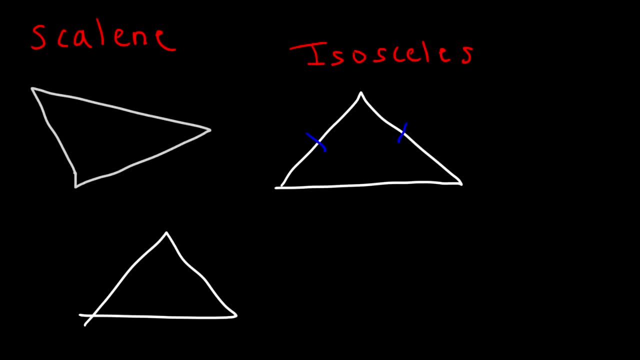 the equilateral triangle, all three sides are congruent. an equilateral triangle is also known as an equal angular triangle, because all angles are congruent as well. whenever the sides are congruent, the angles opposite to those sides are equal to each other as well. so in an 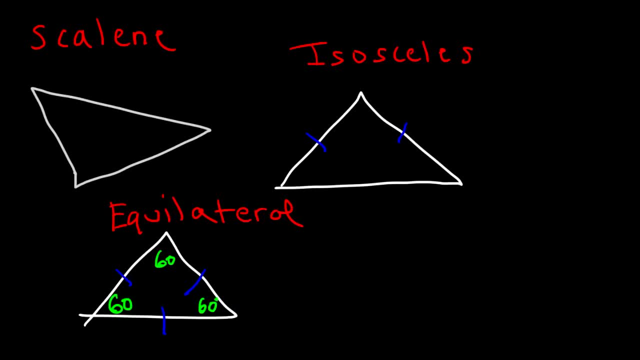 equilateral or equiangular triangle. all angles are 90- I mean at 90- but all angles are 60 degrees and all sides are congruent to each other. now, what I'm gonna do at this point is I'm gonna give you a few triangles and I want you to 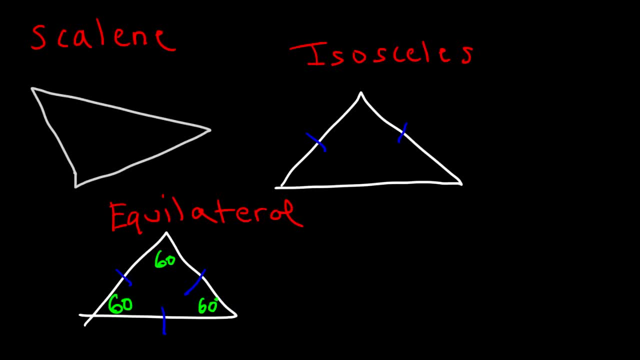 equilateral or equi angular triangle. all angles are 90- I mean at 90, but all angles are 60 degrees and all sides are congruent to each other. now, what I'm going to do at this point is I'm going to give you a few triangles and I want 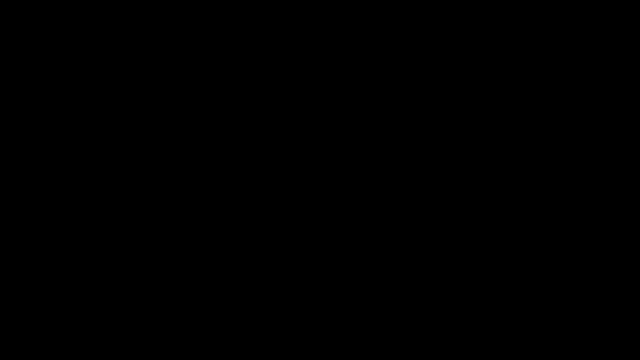 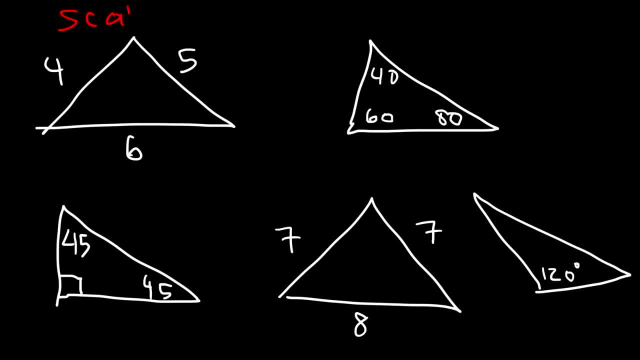 known as a scalene triangle. now what about the second one in the upper right? notice that all angles are less than 90, so therefore this is called an acute triangle. the next one on the lower left: we have a 90 degree angle, so this is a right triangle, also because these two 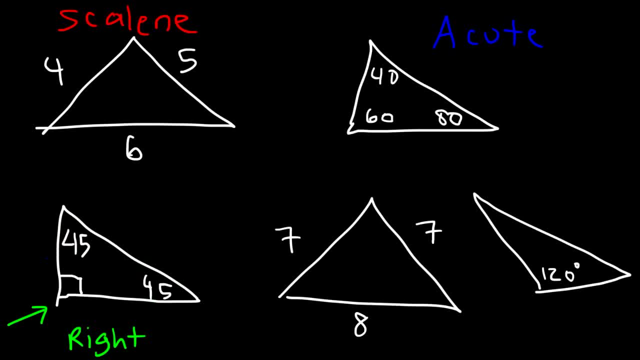 angles are congruent, the sides that are opposite to those angles are also congruent, so this is also an isosceles triangle. so collectively it's called an isosceles right triangle. the next one: we have two congruent sides, so that is just a regular isosceles triangle, and here we have an obtuse angle. so 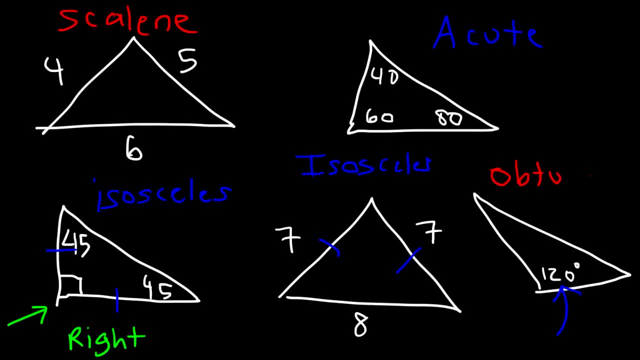 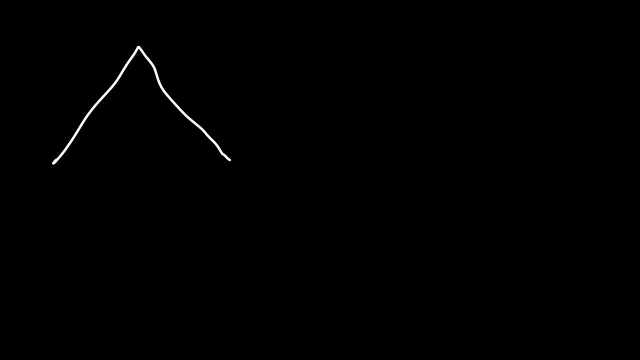 therefore, that is called an obtuse triangle, so make sure you're familiar with these terms, because you're going to see it throughout pre-algebra, or even geometry, depending on what course you're taking now. the next thing that you need to know is that all three of these angles are congruent, so this is an 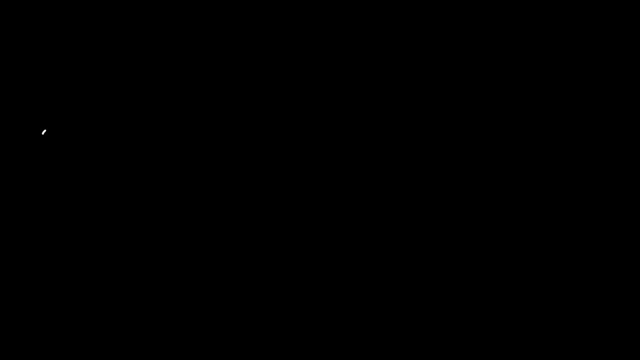 classify them based on what you just learned. feel free to pause the video if you want to. so the first triangle on the upper left side. what is it called? so notice that all three sides are different. so therefore, this triangle is known as a scaling triangle. now what about the second one? 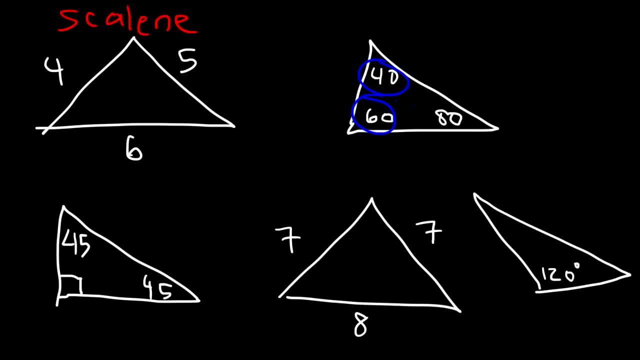 in the upper right. notice that all angles are less than 90, so there's no difference between all three sides. there's not just angle heading relative to every other angle, the angle at prognosis. therefore this is called an acute triangle. the next one on the lower left. 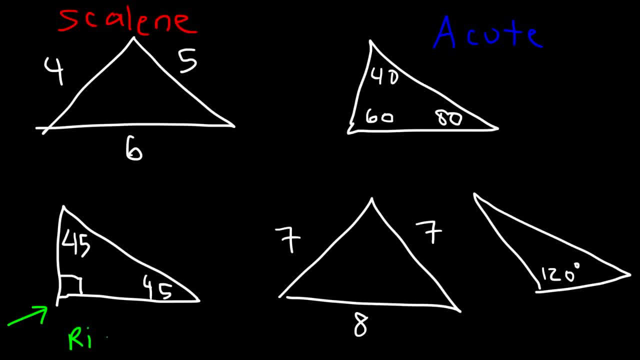 we have a 90 degree angle, so this is a right triangle. also because these two angles are congruent, the sides that are opposite to those angles are also congruent, so this is also an isosceles triangle. so collectively it's called an isosceles right triangle. the next one: we have two congruent sides, so that is. 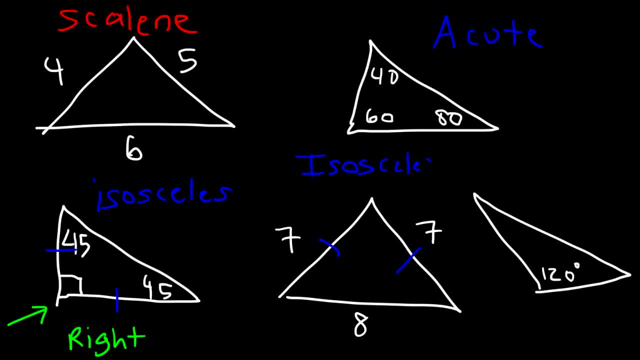 just a regular isosceles triangle, and here we have an obtuse angle. so therefore that is called an obtuse triangle. so make sure you're familiar with these terms, because you're going to see it throughout pre-algebra, or even geometry, depending on what course you're taking. now the next thing that you need: 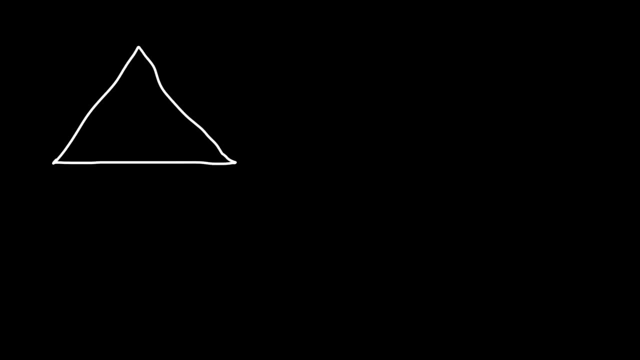 to know is that all three of these angles are congruent. so this is an isosceles triangle and we're going to see that the n of the angles of each of these angles are congruent. so we'll say that on the left side of this triangle, 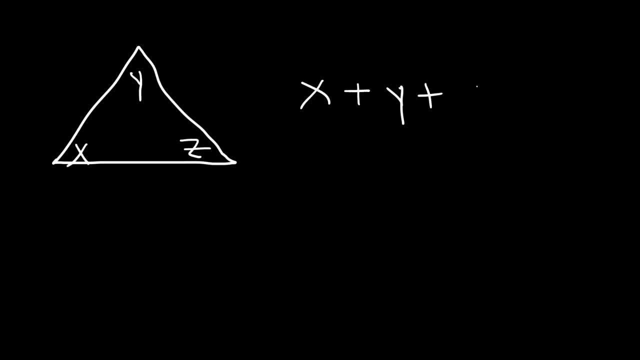 every angles of a triangle must add up to 180. so let's say: this is angle X, Y and Angles e. so X plus Y plus Z has to add up to a hundred and eighty degrees. so knowing that, let's say: if you have this triangle and this is 54 degrees, and 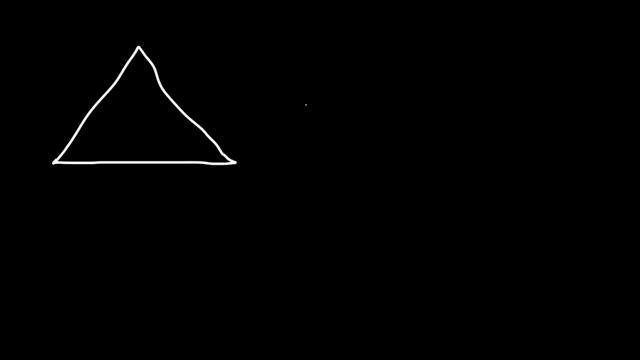 isosceles triangle, and the next thing that you need to know is that all three angles of a triangle must add up to 180. so let's say: this is angle X, Y and angle Z. so X plus Y plus Z has to add up to 180 degrees. so, knowing that, let's say: 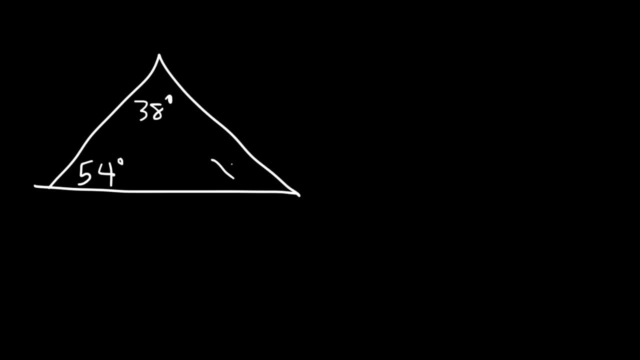 if you have this triangle and this is 54 degrees and this is 38 degrees, and we'll know that the three angles- 54, 38 and the third angle, which is X- they have to add up to 180. so now you could find the value of X. so we just got to do some. 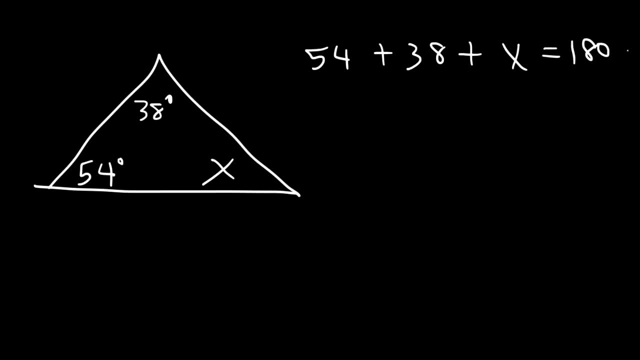 math at this point: 54 plus 38, that's 92. so 92 plus X equals 180. to find the value of X we need to subtract both sides by 92, so X is going to be 180 minus 92, which is 88. so sometimes you may need to find. 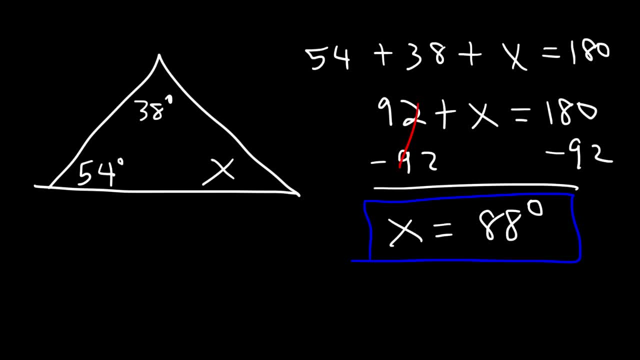 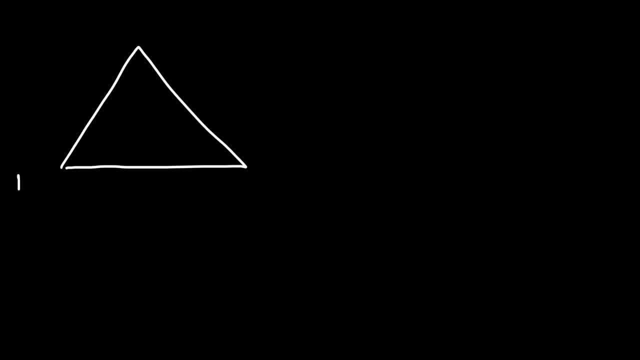 a missing angle, and that's one way in which you can do so is another example. let's say this is angle A, B and C. angle A is 35 degrees, angle B is 4x And angle C is 3x plus 7.. Find the value of angle B. 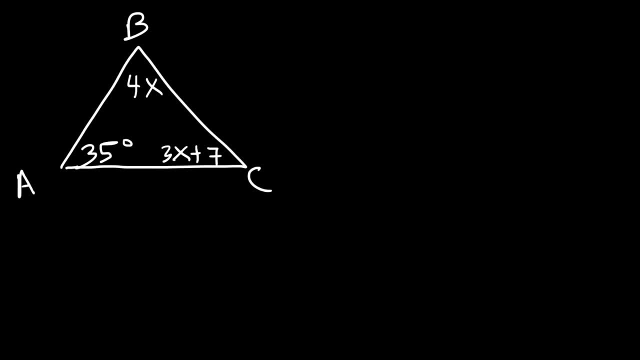 Feel free to pause the video and work on that problem. So let's write an equation. We know that the three angles has to add up to 180.. So angle A, which is 35,, plus angle B, which is 4x, plus angle C, which is 3x plus 7.. 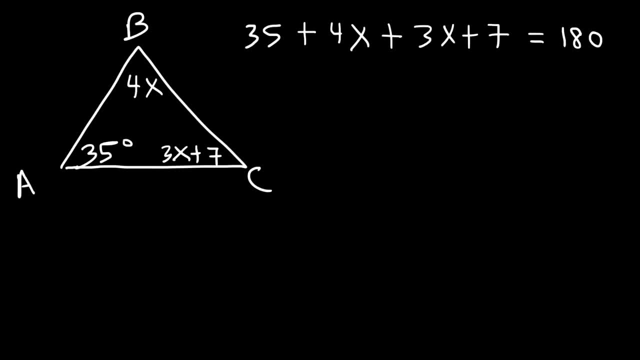 All of that has to add up to 180.. So let's combine like terms 4x and 3x. they add to 7x. 35 plus 7 is 42. So 7x plus 42 adds up to 180.. 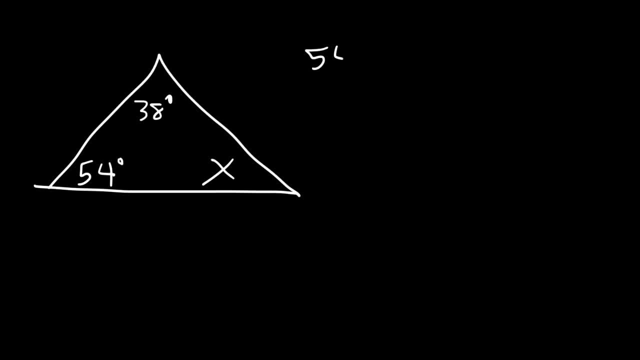 So you know that the three angles, 54,, 38, and the third angle, which is x, they have to add up to 180.. So now you can find the value of x. So we just have to do some math at this point. 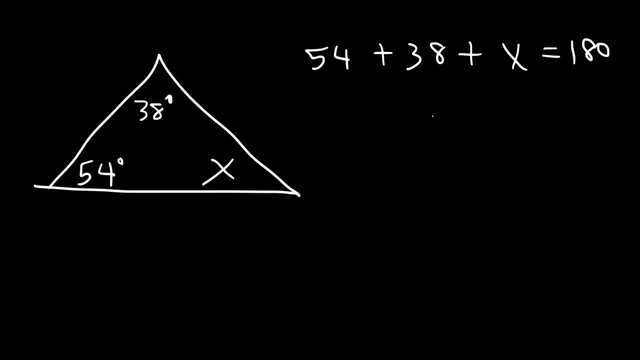 54 plus 38,, that's 92. So 92 plus x equals 180.. To find the value of x, we need to subtract both sides by 92. So x is going to be 180 minus 92,, which is 88.. 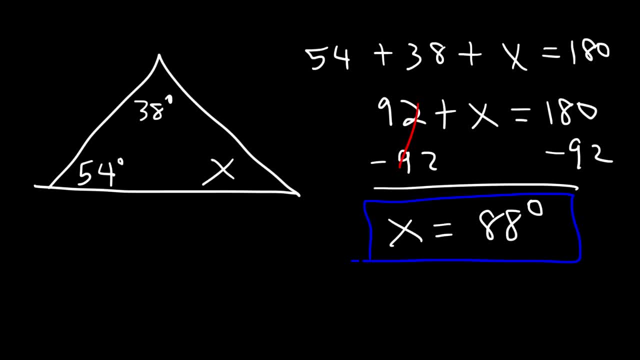 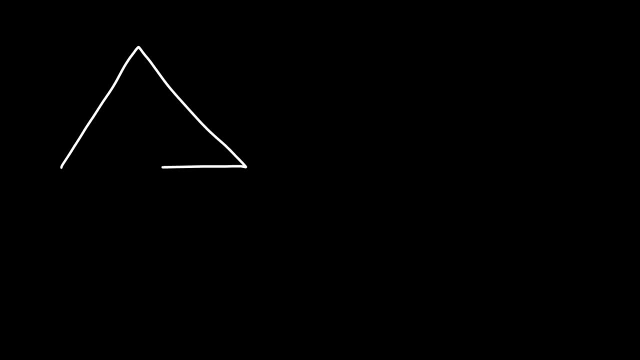 So sometimes you may need to find the missing angle, And that's one way in which you can do so. Here's another example. Let's say this is angle A, B and C. Angle A is 35 degrees, Angle B is 4x. 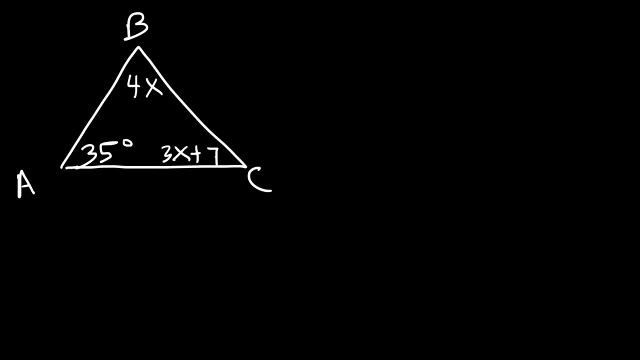 And angle C is 3x plus 7.. Find the value of angle B. Feel free to pause the video and work on that problem. So let's write an equation. We know that the three angles has to add up to 180.. 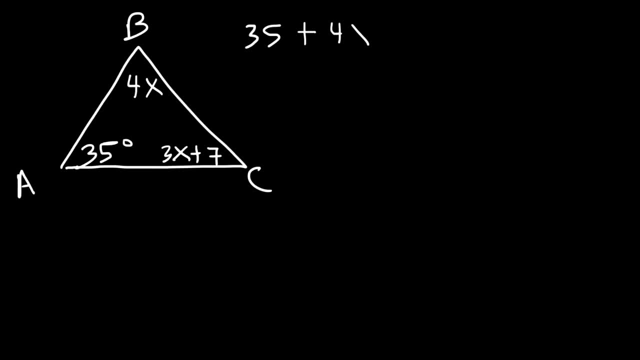 So angle A, which is 35,, plus angle B, which is 4x, plus angle C, which is 3x plus 7.. All of that has to add up to 180.. So let's combine like terms 4x and 3x, they add to 7x. 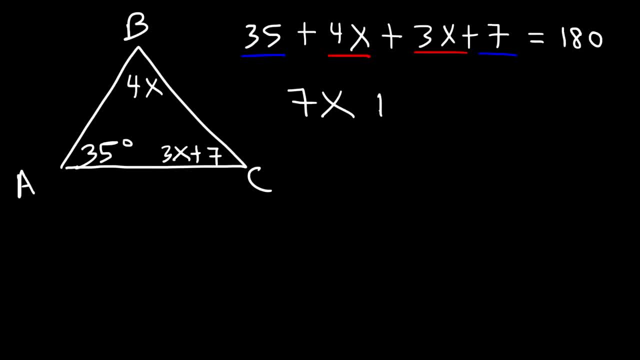 35 plus 7 is 42. So 7x plus 42 adds up to 180.. Now let's subtract both sides by 42.. 180 minus 42 is 138.. So 7x is equal to 138 If we divide both sides by 7. 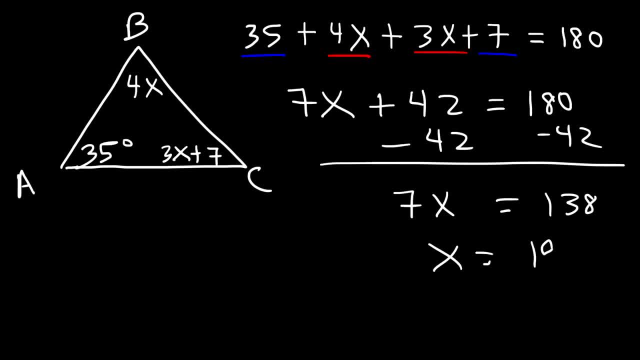 x is about 19.7. Now that's the value of x. Our goal is to find the value of angle B. Angle B is equal to 4x, So we got to multiply 19.7 by 4. It's really 19.71. 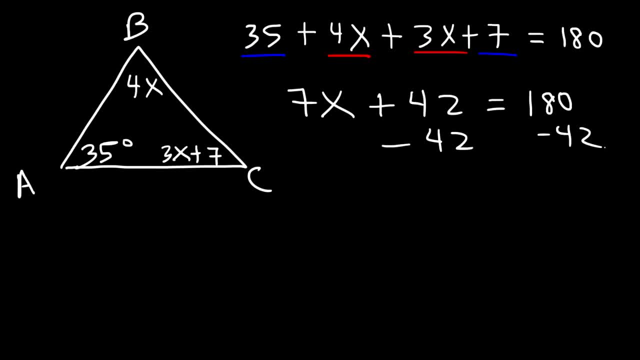 Now let's subtract both sides by 42.. 180 minus 42 is 138.. So 7x is equal to 138.. If we divide both sides by 7, x is about 19.7.. Now that's the value of x. 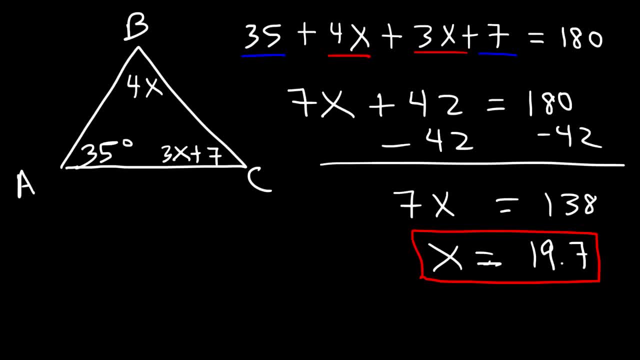 Our goal is to find the value of angle B. Angle B is equal to 4x, So we got to multiply 19.7 by 4.. It's really 19.71. for those of you who want to get a more accurate answer: 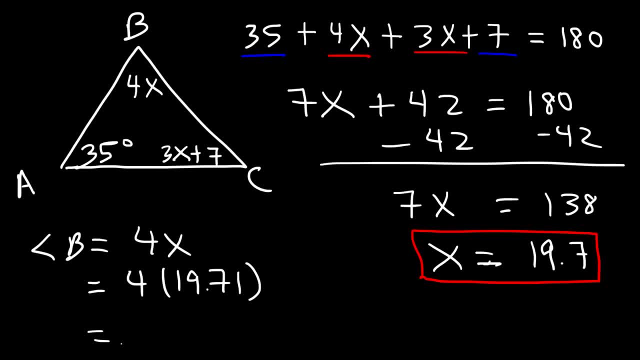 So if you multiply 19.71 by 4, you should get 78.84.. So that's the value of angle B. Now, if you want to find angle C, simply plug it in to 3x plus 7.. So angle C is going to be 3x plus 7, but let's replace x with 19.71.. 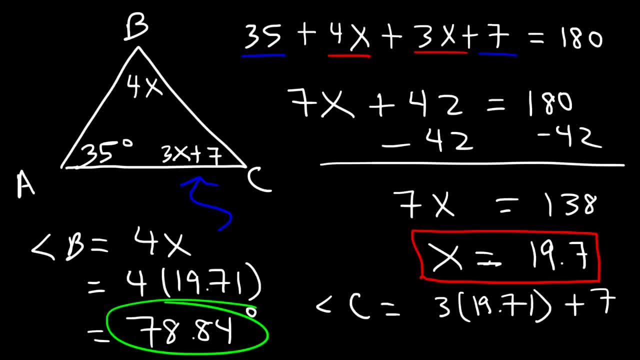 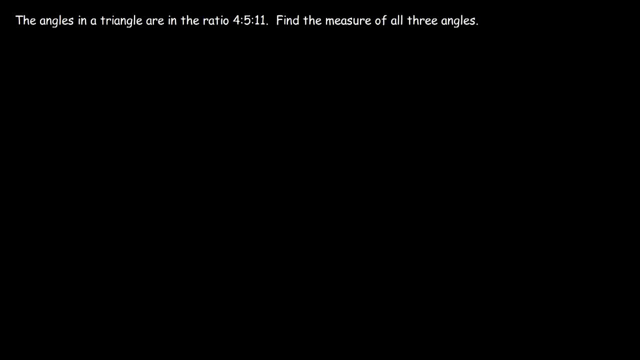 3 times 19.71 is 59.13, and then if you add 7 to it you're going to get this angle 66.13 degrees. so that's the value of angle C. let's try a word problem. the angles in a triangle are, in a ratio 4 to 5 to 11. find a measure of all three. 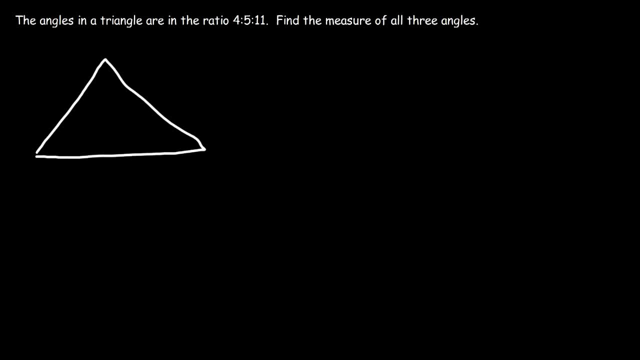 angles. so let's say this is angle a, B and C. so one of the angles has to be 4x, the other has to be 5 and another has to be 11x, because they're in a ratio 4 to 5 to 11. 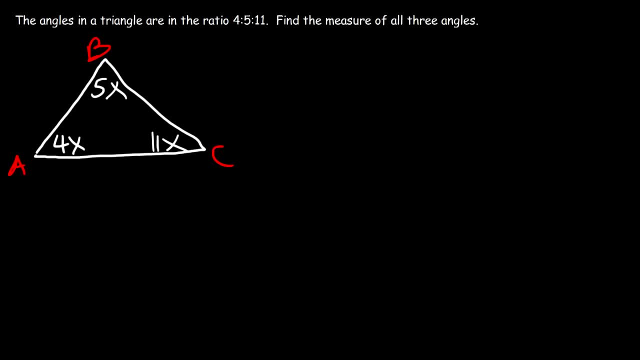 and now we got to do is find the values of a, B and C. so these three angles- 4x, 5x and 11x- has to add up to 180. 5 plus 11 is 16, 16 plus 4 is 20, so these three add up to 20x. so now we need to divide. 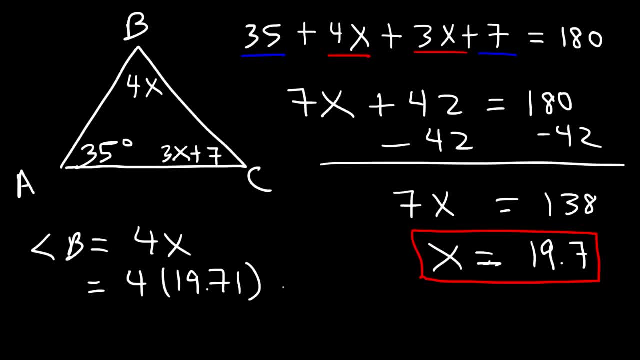 for those of you who want to get a more accurate answer. So if you multiply 19.71 by 4, you should get 78.84. So that's the value of angle B. Now if you want to find angle C, simply plug it in to 3x plus 7. 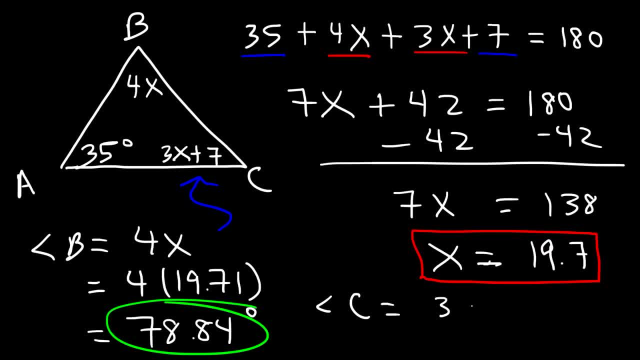 So angle C is going to be 3x plus 7, but let's replace it with 3x plus 7, So angle C is going to be 3x plus 7 with 19.71. 3 times 19.71 is 59.13. 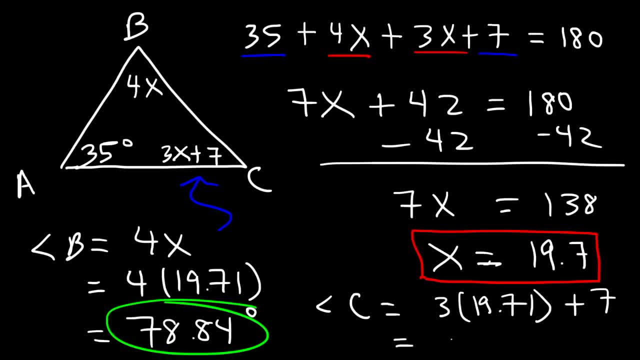 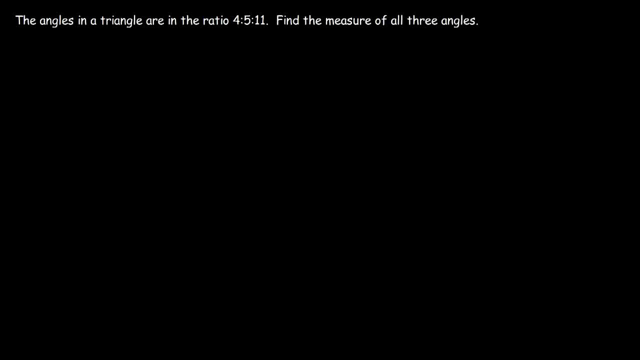 and then if you add 7 to it, you're going to get this angle 66.13 degrees. So that's the value of angle C. Let's try a word problem. The angles in a triangle are in a ratio 4 to 5 to 11. 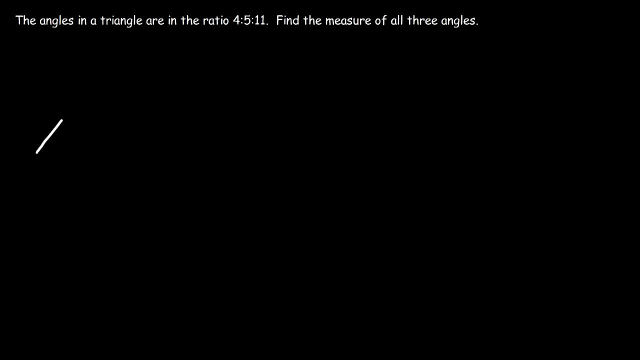 Find a measure of angle C, of all three angles. So let's say this is angle A, B and C. So one of the angles has to be 4x, the other has to be 5 and another has to be 11x, because they're in a ratio 4 to 5 to 11. 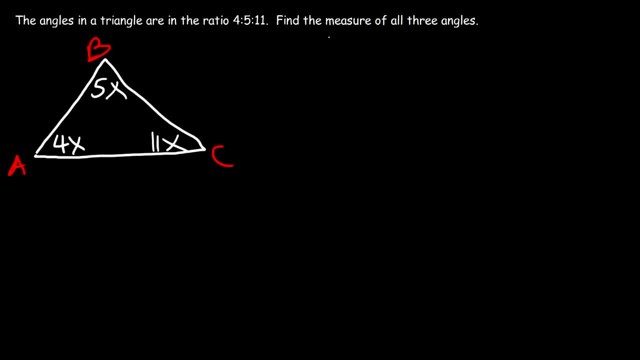 And now all we got to do is find the values of A, B and C. So these three angles- 4x, 5x and 11x- has to add up to 4x and 11x. So these three angles- 4x, 5x and 11x- has to add up to 4x and 11x. 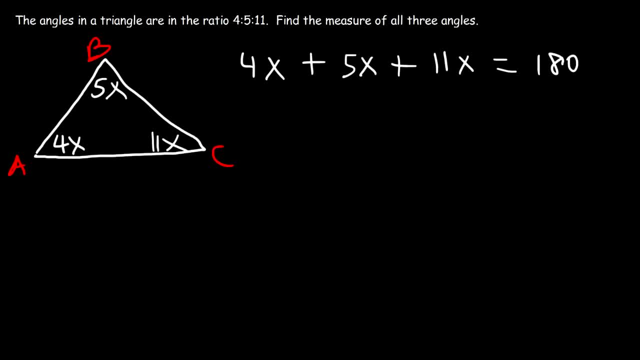 So these three angles- 4x, 5x and 11x- has to add up to 4x and 11x. 5 plus 11 is 16, 16 plus 4 is 20. So these three add up to 20x. 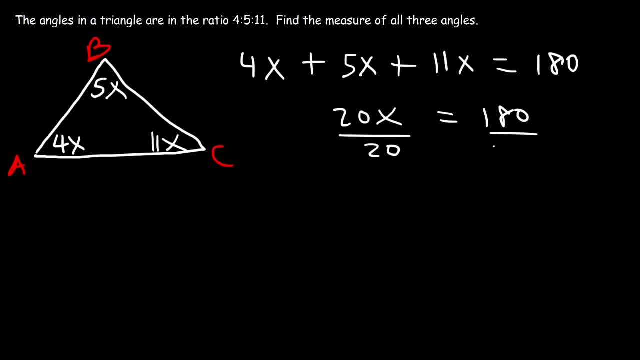 So now we need to divide both sides by 20 in order to find the value of x. So what's 180 divided by 20?? Well, at first we can cancel a 0, So it's equivalent to 18 divided by 2, which is 9. 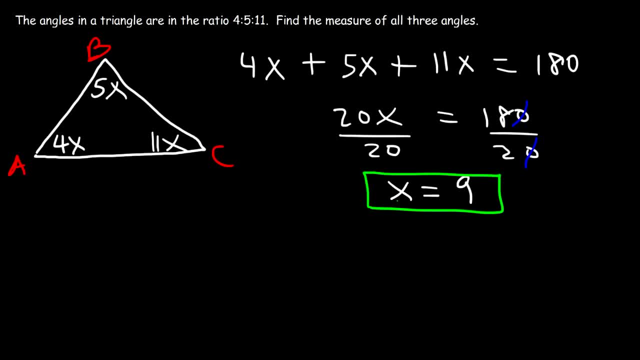 So x is equal to 9. Now that we have the value of x, we're going to find the value of x. We could find the measure of all three angles, So let's start with angle A. So angle A is equal to 4x And x, as we know, is 9.